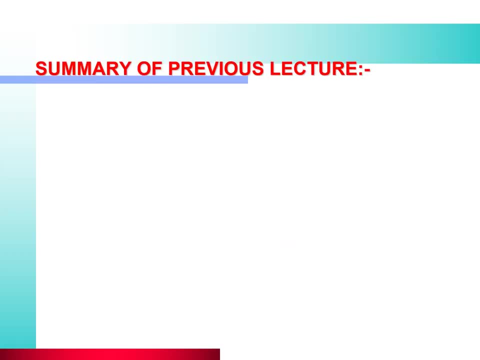 So let us revise the previous lecture. In previous lecture we have learned about metallography, ie the study of observing a sample in a microscope. We have also learned about a sample preparation For clear observation of a sample. we have to make a sample neat and clean. 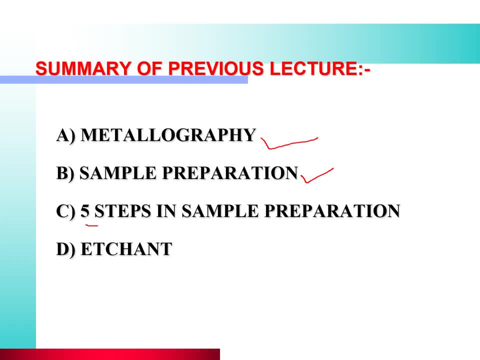 We have also learned about the preparation of a sample. We have also learned about the preparation of a sample. We have also learned about the 5 steps for sample preparation. The 5 steps are: cutting of a sample, then mounting of a sample, then grinding of a sample, then polishing of a sample and last one, very important, ie etching. 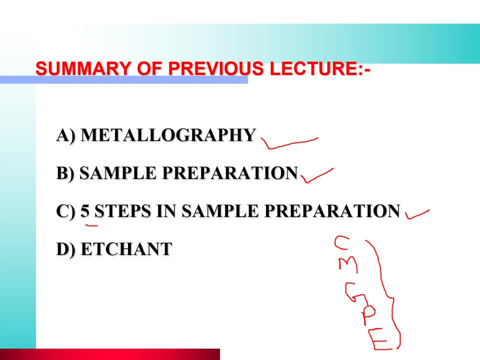 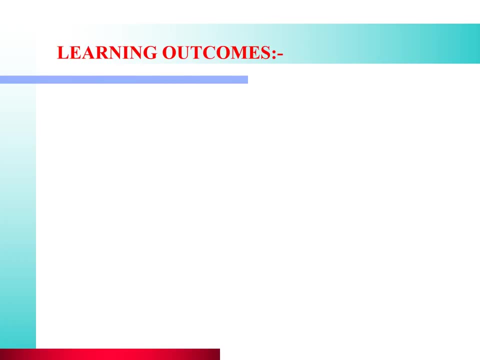 So that 5 steps we have learned for sample preparation. The last topic we have learned is etchant. So there are 2 types of etchants: Dry etchants and wet etchant. Learning Outcomes: After completion of this lecture, you are able to: 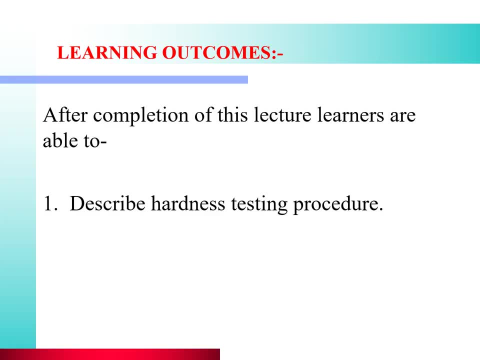 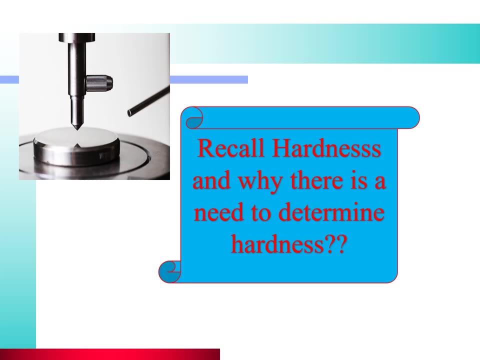 Describe hardness testing procedure. Choose relevant hardness tester based on given situation. So before starting our lesson, we would like to remind you that we are not going to be doing a video on hardness testing. We are learning about the find, the definition of hardness. 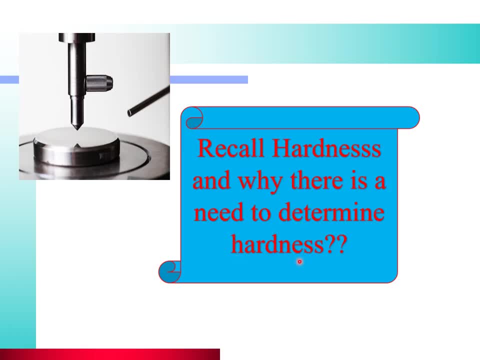 Now you have to know why we are taking a decision on the hardness of the material. We have few examples of this definition. It is clear that in this lecture I would like to ask one question. In previous lecture we have learned about this term. 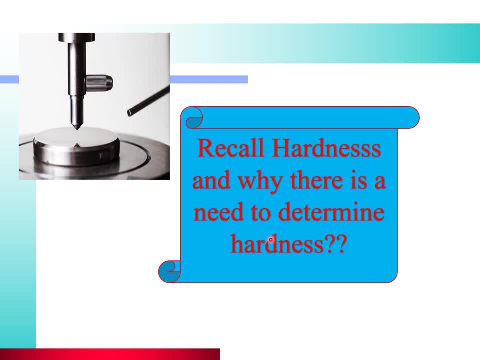 long prail. thats a hardness right. recall the definition of hardness, why there is a need to determine the hardness by a question you have been given to this definition, Is not it? Okay, just remember it. calculate karna chahiye. iske baare mein thoda socho video ko pause kijiye aur thoda sochiye. 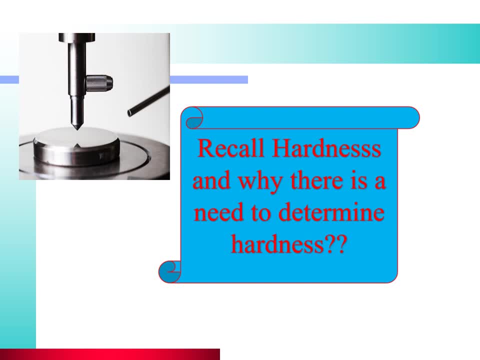 achcha, toh kuch socha aapne hardness ki definition. humne iske pahle lecture mein padhe hai: hardness is the property of material to resist scratching, penetration and wear hume. agar kisi material ke tools banane hai, toh unki hardness jyada chahiye hoti hai. aur. 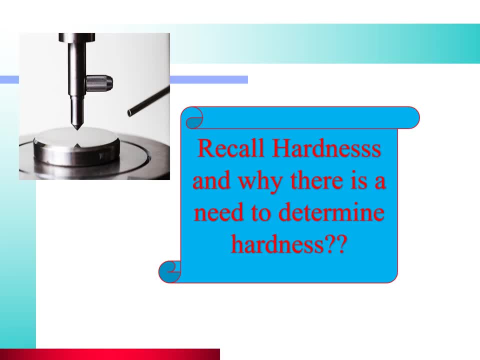 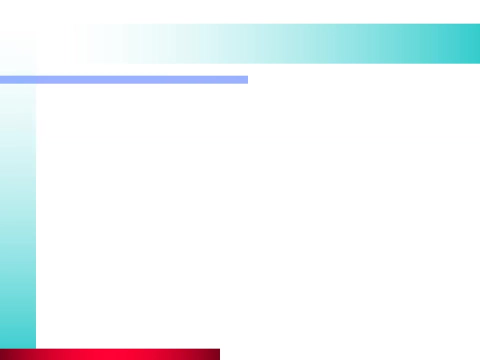 hume agar bahut saare materials ki hardness compare karna hai. hardness is the property of material to resist scratching, penetration and wear. toh sab ki hardness ko calculate karna hoga, taaki hum desired cutting tool material select kar sake. isliye hume hardness testing karna jaruri hai. toh dosto hum types of hardness testing ki. 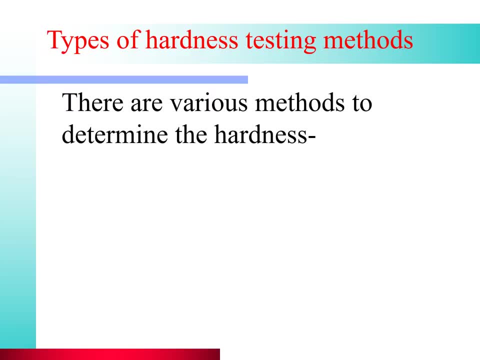 hoga ka sy. whereas hardness is the property of material to resist scratching penetration. remarkable neこの software to consider sゴse kaji main В sector pits mereka has are various methods to determine the hardness. there are various methods to determine the hardness. first, brinole hardness test. first brinole hardness test. 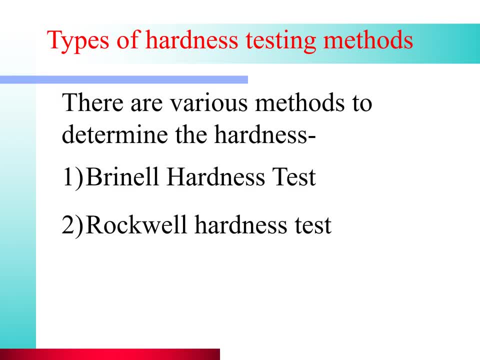 Rockwell hardness test. wickers hardness test. manterai hardness test. wickers hardness test. wickers hardness test. shamish test. wai test asselfine. __. walter inshile test uan himell. let us begin with our first hardness test. ools this control be insuch ziem test perspiras ki. 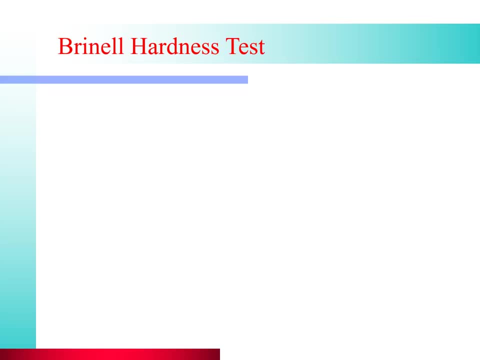 ourqist hardness test. this control be this is the signature method of yourيف Moshe bhr WA. assess two something fika of your hard weather: Vernon high chamskade. Brinell hardness test. this diagram you are seeing on the slide is the actual Brinell. 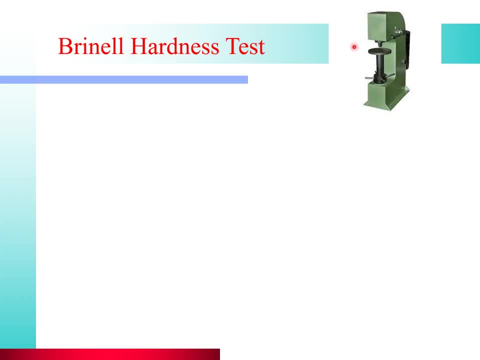 hardness tester which is available in our laboratory, and we have to do a lot of hardness test. in this diagram I have told you about the main components of Brinell. hardness test like this is a lever. with the help of this lever, we can apply the loads of this hanger. 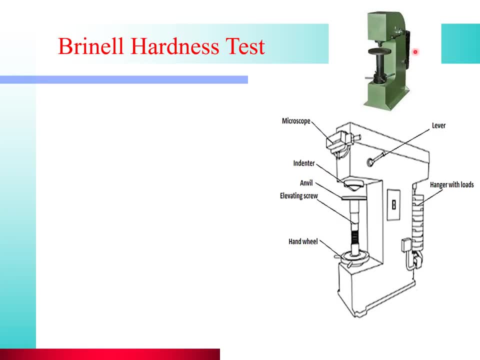 as you can see here. here is the lever and here is the hanger in which the weights are placed. here you can see a handwheel. as we rotate this handwheel, the elevating screw moves up and down. this elevating screw has a platform attached to it. this elevating 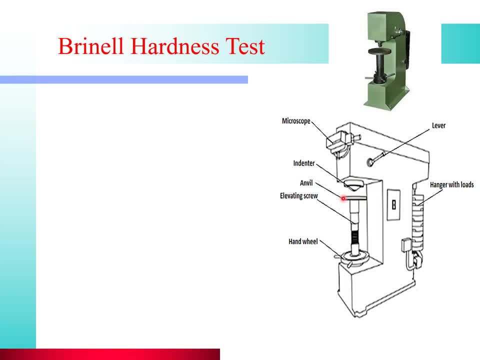 screw, and this is the platform. this platform is called anvil and on the anvil we place a sample. So this is an anvil, and on the anvil we place a sample. So this is an anvil, and on the anvil we place a sample. 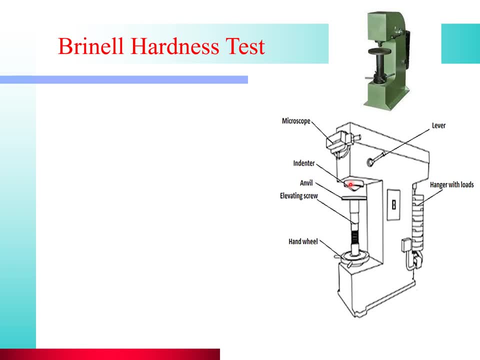 So this is an anvil and on the anvil we place a sample. Now in this diagram, the intender which you see here. the same way we apply the load to the weight and press the lever, this intender makes an impression on that sample makes. 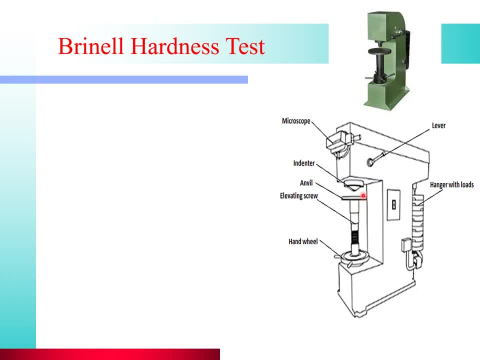 a mark and we can see that impression in this microscope and through that we can do the Brinell hardness test of the sample which we took. So this is an intender which you can see here. this is the intender which you can see. 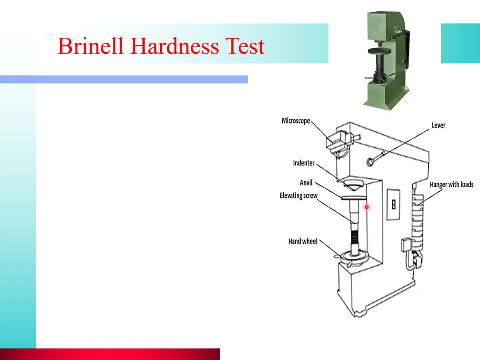 on the anvil. and on the anvil we place a sample and can find out its BHN, Brinell hardness number. Brinell hardness test is done specifically for those materials whose surface is rough or coarse, like casting and forging. 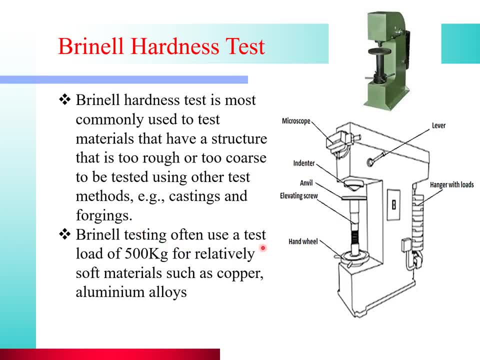 For Brinell hardness test. if we want to test soft material like copper and aluminium, then we have to apply weight or load of 500 kg. If we want to observe or test hard material from Brinell tester, then we have to apply weight or load of 3000 kg. 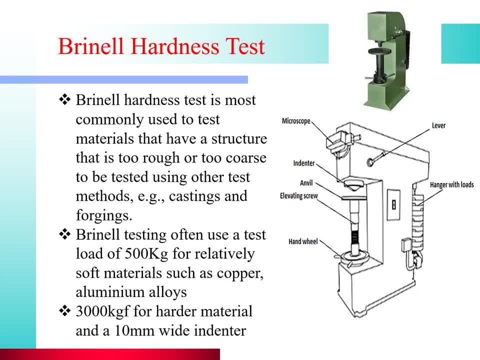 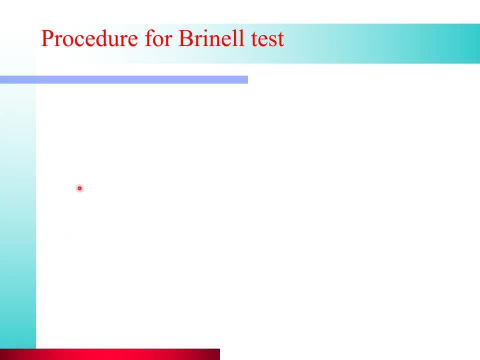 If we want to observe or test hard material from Brinell tester, then we have to apply weight or load of 3000 kg. Now we will see how to perform Brinell hardness test on the machine. Select the proper size of a ball and load to suit the material under test. 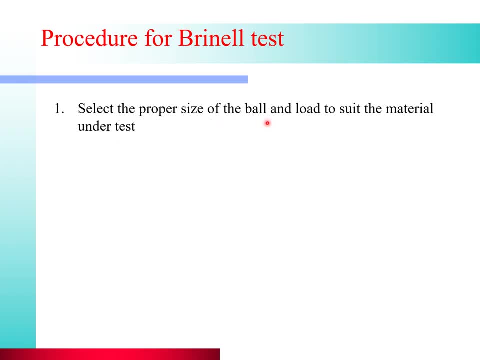 First of all we have to take ball type intender And which material, which load we are applying for test. we have to select that Clean the test specimen to be free from any dirt and defects. We have to clean the sample properly. 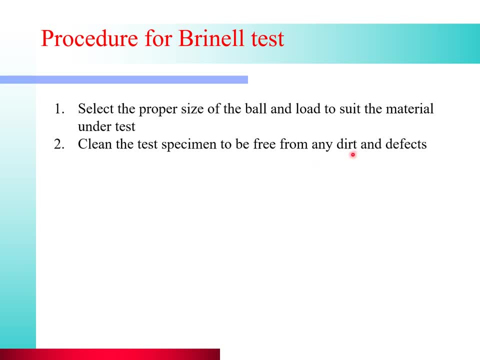 so that we can remove the dirt on it. Mount the test piece surface at a right angle to the axis of the ball intender plunger. We have to take right angle, ie 90 degree angle, and we have to mount the work piece under the ball intender. 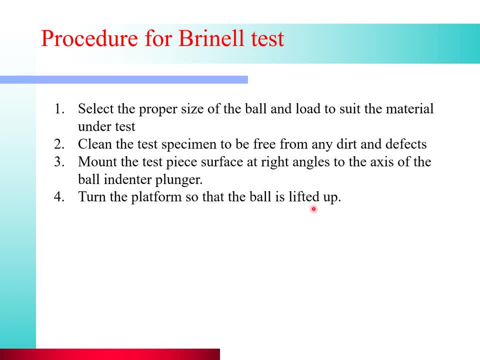 Turn the platform so that the ball is lifted up. We have to turn the platform with the help of the handwheel shown So that the ball intender goes up a little By shifting the lever, apply the loads and wait for some time. 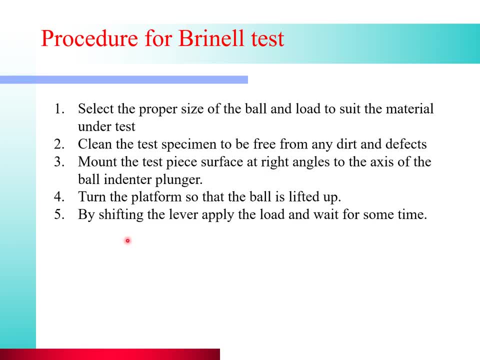 As the ball is lifted up, we have to apply the load with the help of the lever and wait for some time. Release the load by shifting the lever. We have to release the load by shifting the lever. Take out the specimen and measure the diameter of the intender by means of Brinell microscope. 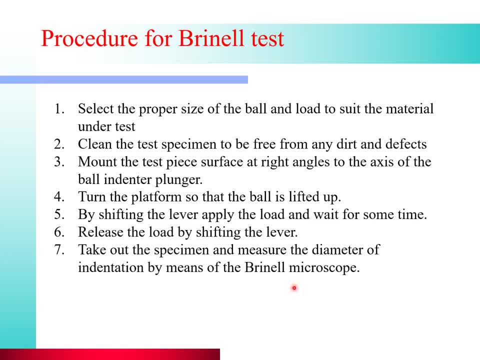 We have to take out the sample or the specimen And through the microscope we will get the mark of the intender. This is the sample. We will get a mark like this Right, So we have to check the diameter of this mark. 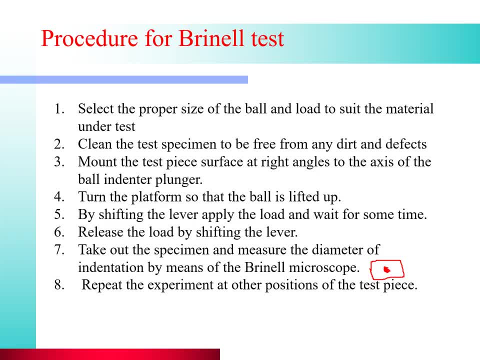 With the help of Brinell microscope. Repeat the experiment at other position of the test piece. We have to take the marks at 4-5 positions like this And we have to take out its diameters, Then calculate the value of Brinell hardness number. 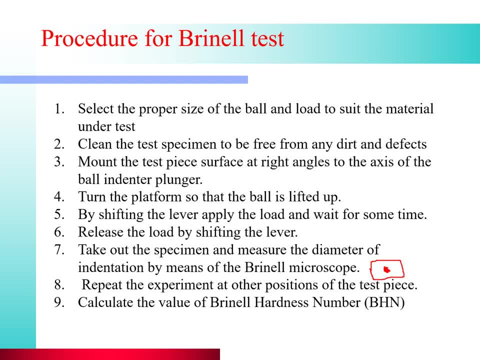 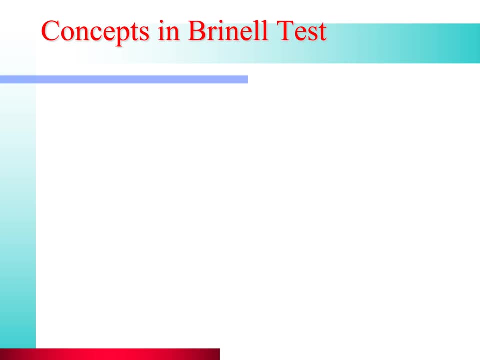 There is a formula in which we have to put up the values And then we can find out its BHN number, As we have seen in the procedure. Now we will see the concept. See this animation, This yellow color that you are seeing. 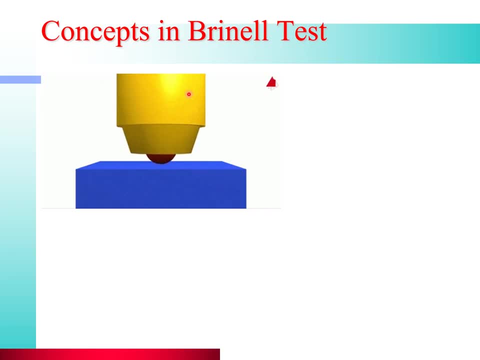 This yellow color is a plunger And in this plunger we have a red color that is a ball type intender. This is our work piece As we apply the load. This ball type intender will mark on this sample Which you are seeing. 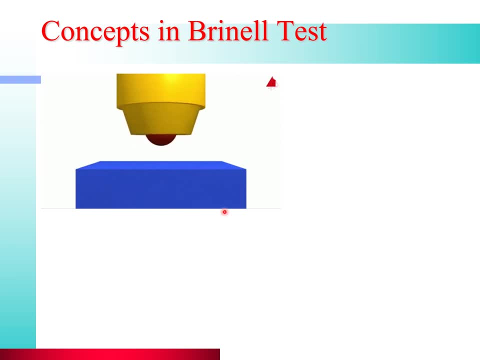 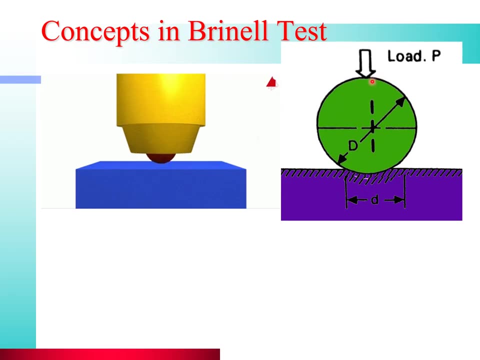 Right, friends, See, here we have put the load of P. This ball will be the diameter of this ball type. intender, That value is the capital D. We know this, Like. this is a ball. We know its diameter As it will come on the sample. 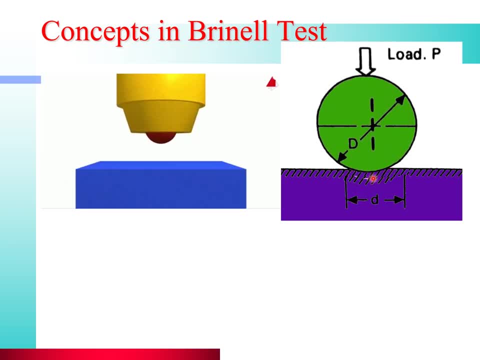 So it will give us some diameter here. Right, friends, We will get some impression here. We will check the diameter of that impression with a microscope. That small d is the diameter of intender. It is the diameter of intender. So this is the formula. 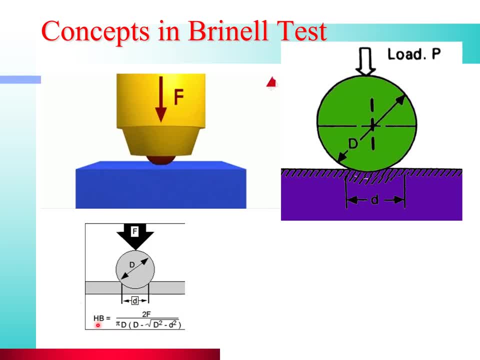 This is the formula to calculate the BHN number, That is the formula 2f divided by pi d bracket, capital D minus under root d square, minus small d square. So, friends, here we do not know the value of f, So this f is 30.. 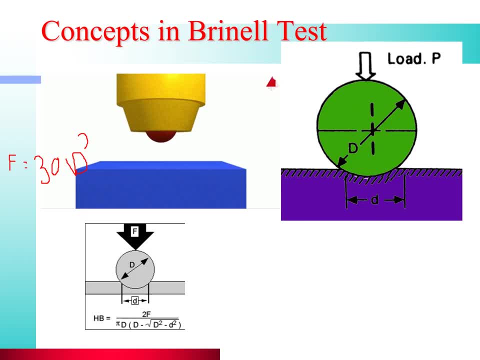 We have to take 30 into d square, Capital D square, 30 into capital D square. So if the diameter of this ball is 10 mm, So 10 square is 100.. 100 into 30 is 3000.. 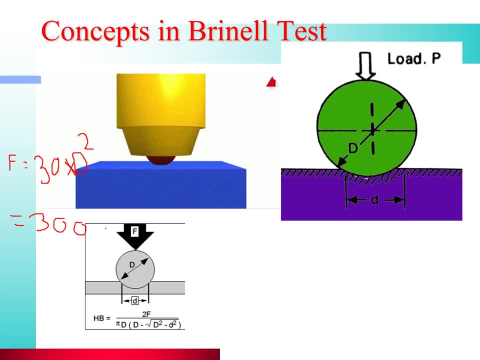 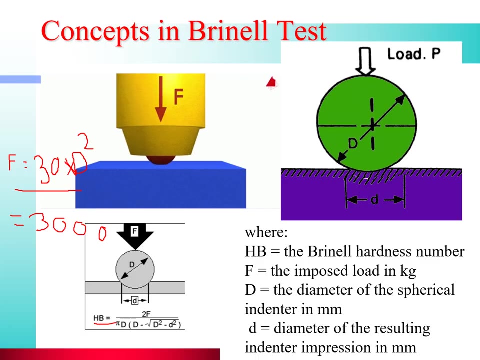 So 3000 kg, we have to put the load here. So from where you have to take f 30 into diameter square, We will put it here. So we will get the BHN number, HB or BHN, the Brinell hardness number. 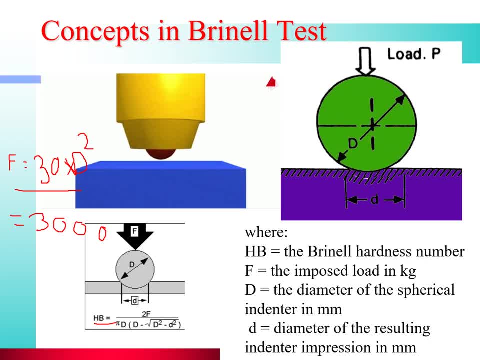 F is the imposed load in kg. D is the diameter of the spherical intender And small d is the diameter of resulting intender impression in the mm. So this formula is very important. It comes in the exam every time As the formula comes. 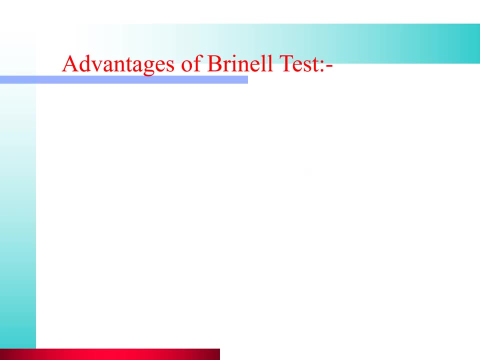 So let us discuss the advantages of Brinell test. The flat, irregular metal surface does not affect the Brinell hardness test. As we saw in the introduction that the surface of the castings and some of our materials of forging is rough, We can check them with Brinell test. 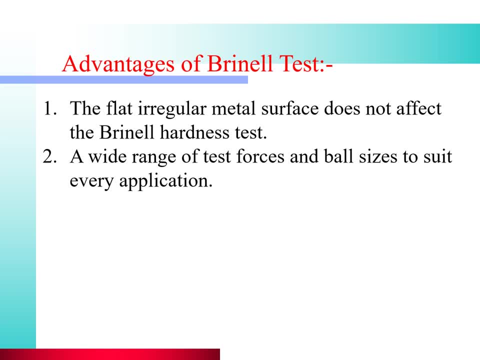 A wide range of test forces and ball sizes to suit every application. We have many intender ball sizes. We can use different forces to get the BHN number And this test is non-destructive. That means if we do intendation on the sample. 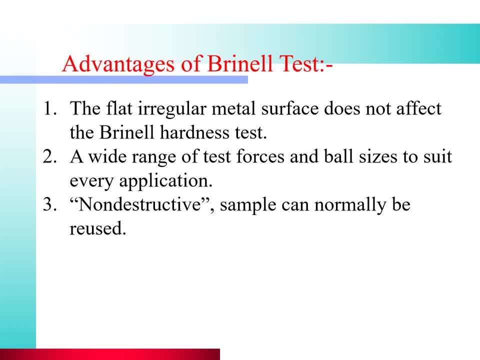 Then the sample is not that bad. We can use that specimen again and again. This hardness test is less sensitive. Intendation made on the sample can be seen and measured under microscope or eyepiece. Whatever intendation we got there, We got a mark. 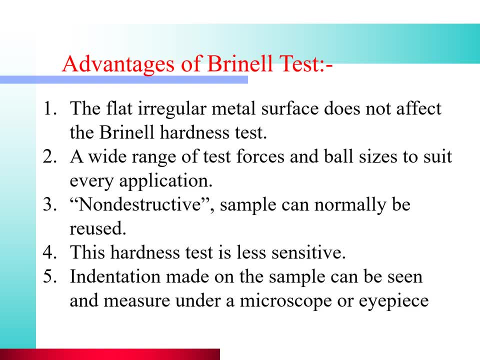 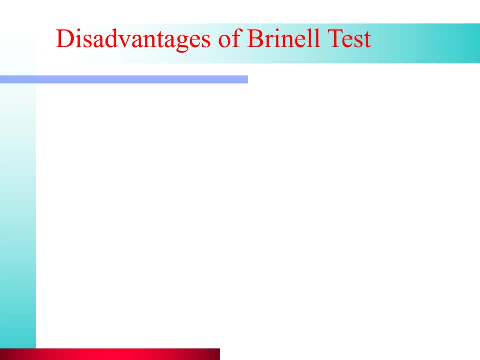 We can easily observe that with microscope. Okay, So let us discuss about the disadvantages of Brinell test. The main disadvantage of this test: that is not suitable for small size object. due to large intender impression, We cannot use this for small sample. 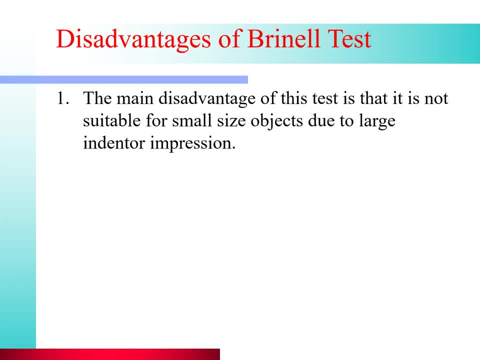 The small size objects Because the impression of intender is little big. The next drawback is Brinell test is in need to optically measure the intender size. This requires that the test point be finished well enough to make an accurate measurement. 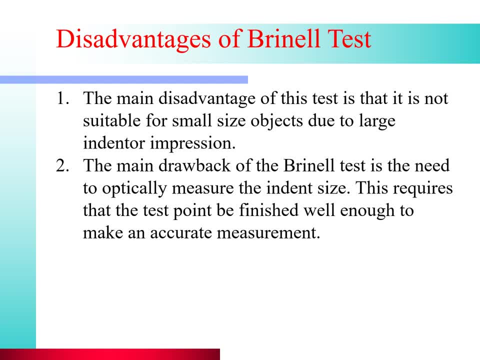 See, Sample preparation plays a very good role here. If your sample is well prepared, Then only we will be able to take the impression easily from the microscope. If we did not prepare the sample well, Then Brinell test will not work. 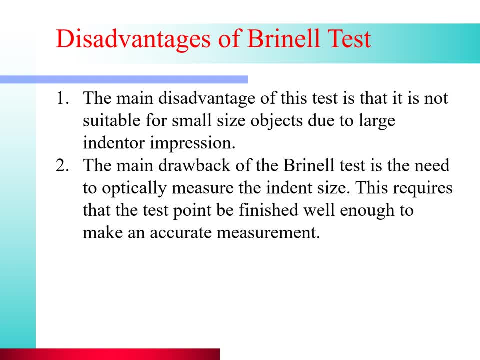 So we have to keep in mind that we have to take the sample neat and clean. This test is very slow. It may take 30 seconds. Not counting the sample preparation time, It will take 30 seconds, But it will also take time to prepare the sample. 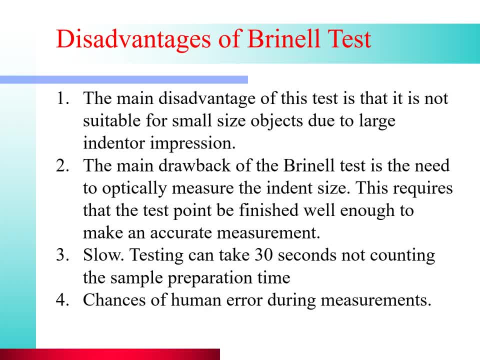 So this test is quite slow. Chances of human error during measurement. Human error may occur when we are going to see the diameter of the intender from the microscope, So it should be measured accurately, Otherwise our Brinell number will be wrong. 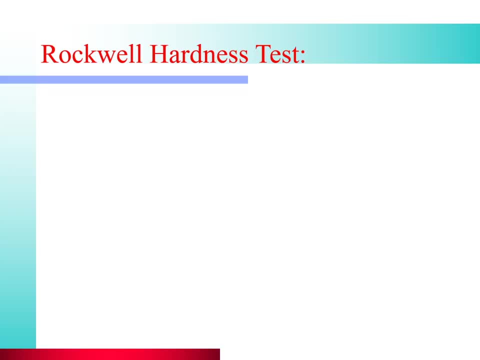 The next hardness test is Rockwell hardness test. This figure on the slide is the actual Rockwell hardness tester Which is available in our laboratory. In this diagram I have tried to show you some components of this machine. Like here I have given you a loading device. 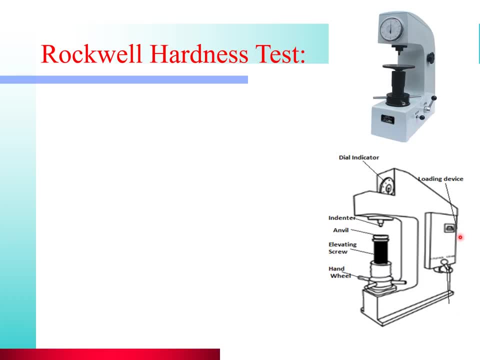 Through this loading device, we can apply minor and major loads. This is the handwheel. Like in the previous one, This is the elevating screw. This is anvil. This is intender. All these are similar to Brinell hardness testers. 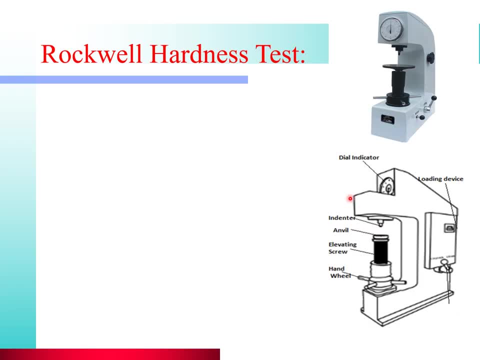 But in Brinell there used to be a microscope. But there are changes in Rockwell. Here there will be a dial indicator. Keep it in mind. In Rockwell hardness tester there is a dial indicator Which will give us our number directly. 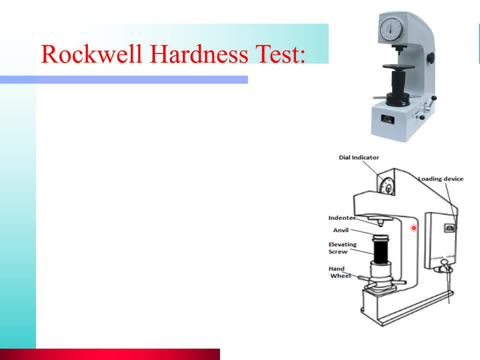 If we do the hardness test of the sample, Then the HRC number will tell us the dial indicator directly. So here through the microscope, There is no need to find out the diameter of the intender. Rockwell hardness tester present. direct reading of hardness number. 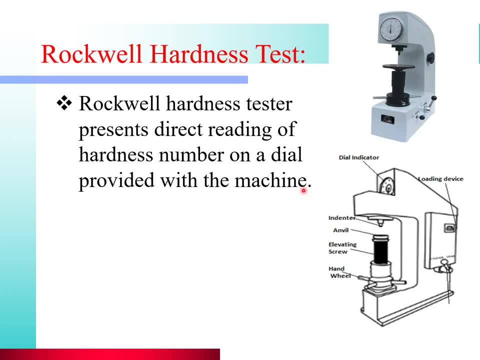 On a dial provided with the machine. Like we just told you, This gives us the direct reading of hardness number, Called this dial indicator. Principally, this testing is similar to Brinell hardness testing. Testing is similar to Brinell hardness testing. 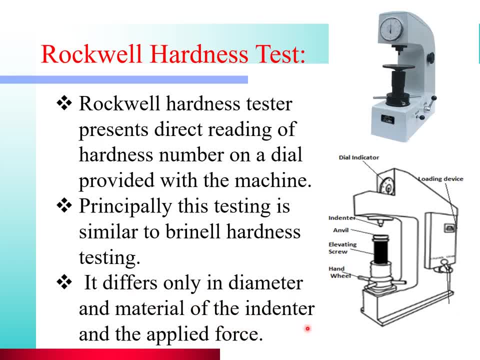 It differs only in diameter and material of the intender And applied force. There is a slight difference here: Which intender we have to take, How much diameter we have to take And how much force we have to apply. These are different in this Rockwell hardness test. 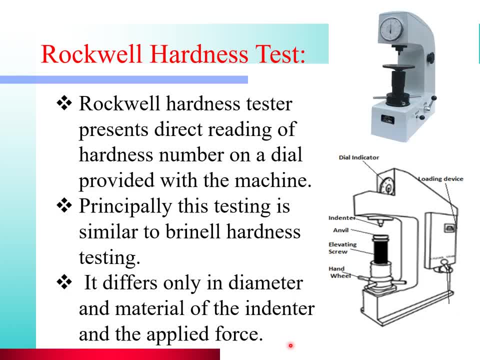 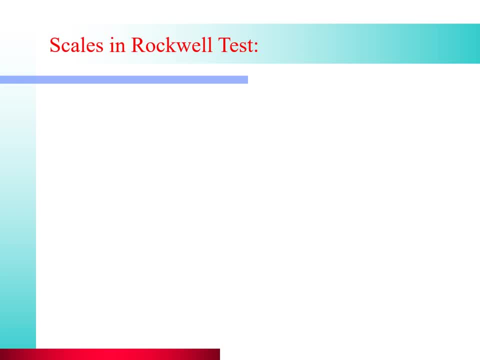 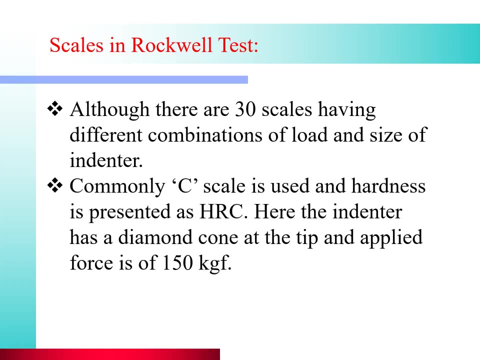 Rest of the process is similar to Brinell In Rockwell test. the concept of scale is very popular. Rockwell scale has 30 scales available, Which depends on the load and size of the intender. Commonly, C scale is used. 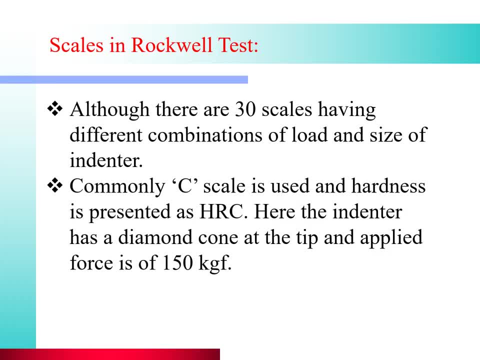 And hardness is presented by HRC. The most popular scale is. The most popular scale of Rockwell test is HRC. Here the intender has a diamond cone at the tip And applied a force of 120 kg. We have to keep in mind that. 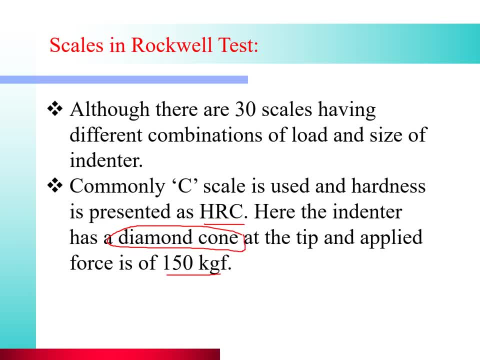 Diamond cone is used in C scale in HRC And 150 kg force is applied there. The soft material is rated in B scale. Here we take intender ball type. In intender B scale we take ball type Which has a diameter of 1 by 60 mm. 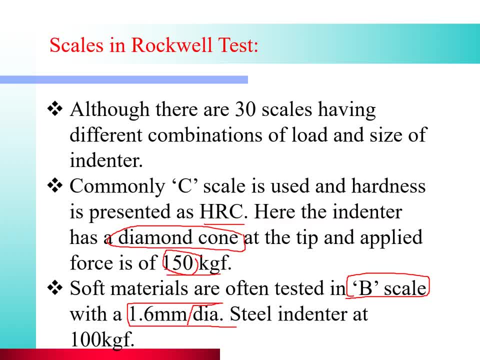 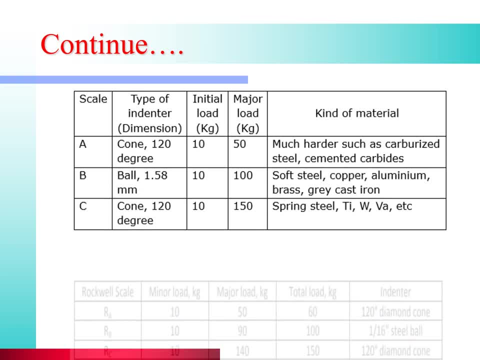 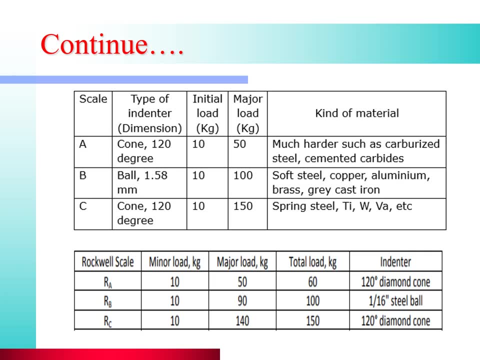 1.6 mm And we apply load of 60 kg there. Now we have a little difference in ABC scale. Let's see the difference in ABC scale. This is a very important table. You will get two questions in the exam. 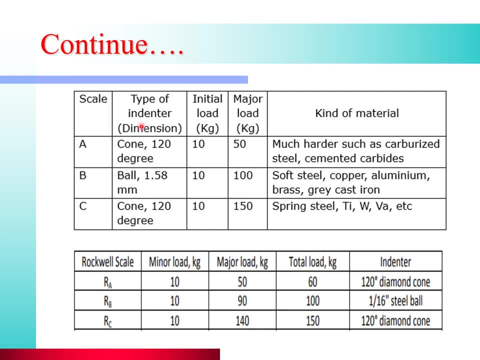 We have just studied C scale. In C scale, which intender will we use Cone type intender, Its angle will be 120 degree. Is it correct? C-type intender- Cone type intender Its angle is 120 degree. 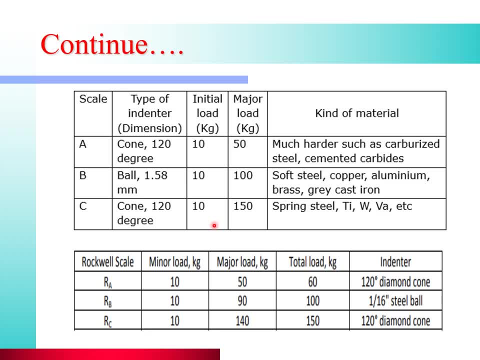 We call minor load or initial. Minor load is called initial load. We will apply that of 10 kg, Is it correct? And major load will be 150 kg. So minor plus major, 10 plus 140, total load is 150.. 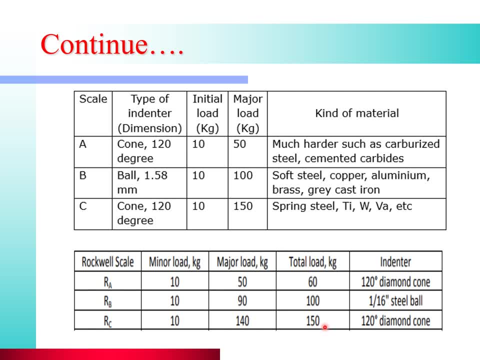 So you have to keep this value in mind: 150 for C-type scale, And this C-type scale can be used for spring steel, titanium, tungsten, vanadium. For B, we will use ball type intender. Its diameter is 1.58.. 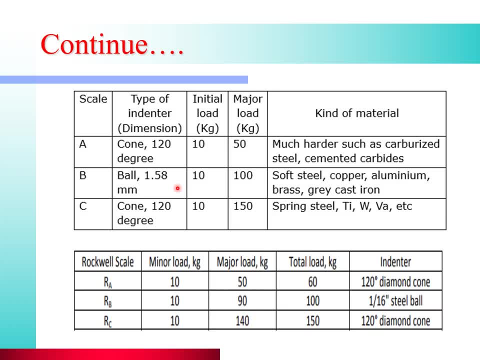 So 1.58 is around 1.6.. Is it correct? So we can take 1.6 mm also. Or 1 divided by 16 inch, 1 divided by 16 inch. So 1 inch means 25.4 mm. 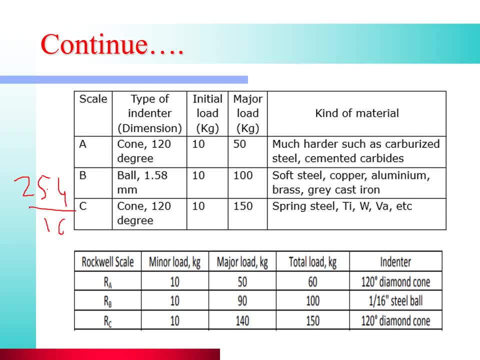 Is it correct If we divide it by 16.. So what value will we get? We get 1.58.. So you have to remember two things: in B scale, If you ask in mm, Then 1.58 or 1.6 or 1 divided by 16.. 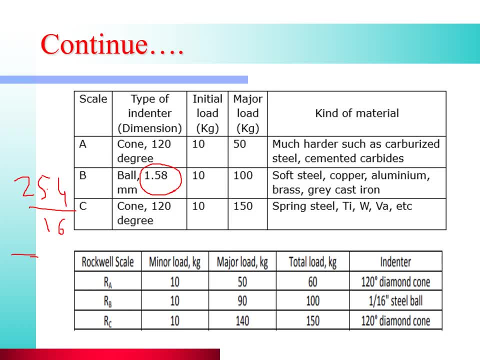 1 divided by 16 is inch, But if you want to convert it Then you will get 1.58. only B scale is used for soft steel, copper, aluminium, brass, grey, cast iron In which minor load is 10 kg. 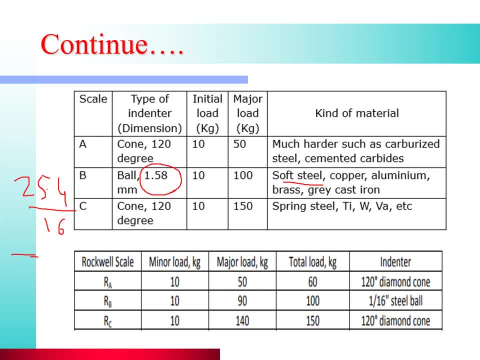 See, in all three, minor load is 10 kg, Major load is 90.. The total weight is 100.. Is it correct? Total weight is 100.. So you can see it here. So in B scale you have to remember 100.. 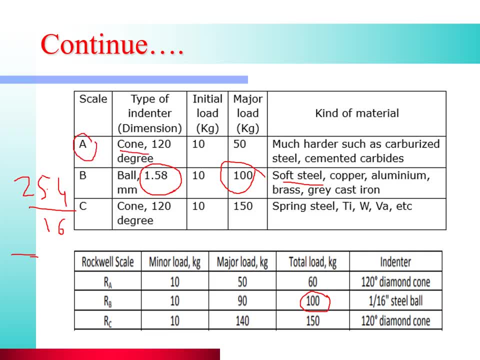 Then, in A type scale, we will use cone type intender. Its angle will be 120 degree, Is it correct? And initial load we are going to take 10.. Major load we are going to take 50. And total load will be 60 degree.